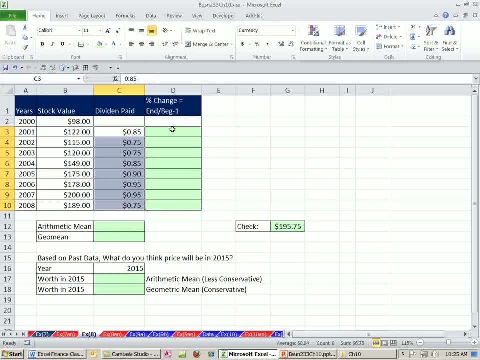 We want to take some stock values and dividends, estimate our period returns and then figure out what the two means- are arithmetic and geo mean- and then estimate what the stock may be worth in the future. All right, as we've done many times in this class. 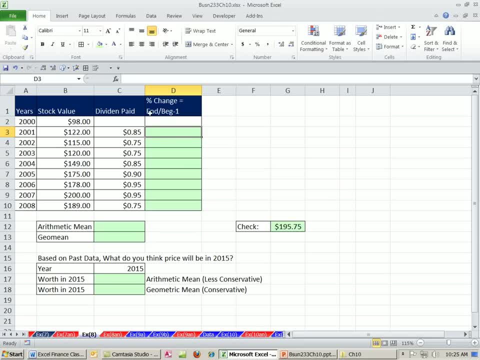 and in this chapter we're going to take our ending value. We need to figure out the percentage change, So the ending value divided by begin minus 1.. Well, we just need to take into consideration dividends. So the ending value will be: hey, the stock after one year. 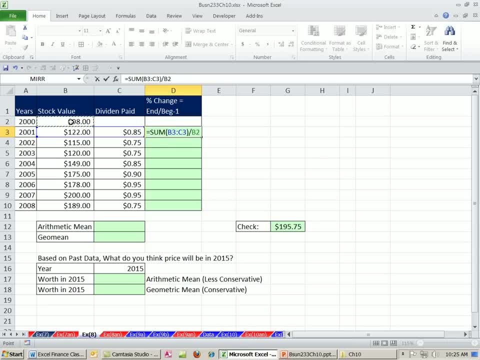 plus the dividend they pay, That'll be the end value compared to begin value minus 1.. That formula- relative cell references- can be copied all the way down. Come down here. you can see the formula works just fine. Now let's calculate our average. 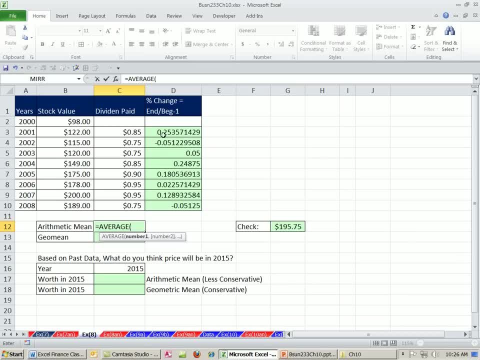 The arithmetic mean. we'll use the average function, And the average function arithmetic mean will give us a slightly high number: The geo mean. now what we need for an input for geo mean is 1 plus this, 1 plus this, 1 plus this. 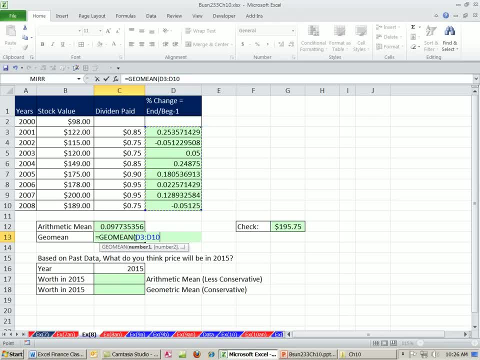 Well, we don't have that. We're just going to use the straight numbers And then this is an array of numbers And we're going to add 1.. When doing array formulas, an operation on this array plus one, will be added 1 to each one of these. 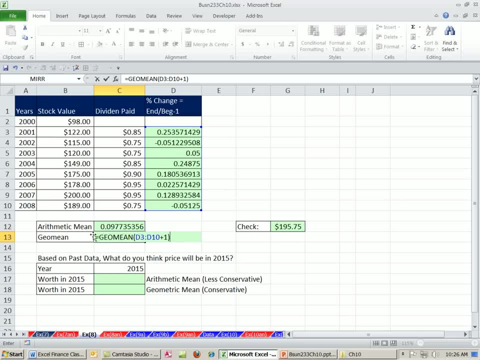 Now, as we saw in the last video, that's an array formula And Excel has to put the array formula into the cell in a special way. So the way we're going to do it is this: Why the SUMPRODUCT, Now SUMPRODUCT, this right here. if I highlight this, 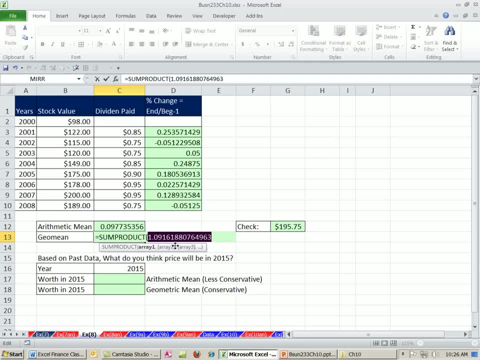 and hit the F9 key. you can see. that's the answer. we're looking for Control-Z, But because this is an array, we can't just enter it into the cell. We're going to put it inside the SUMPRODUCT, because the SUMPRODUCT function has an argument that actually 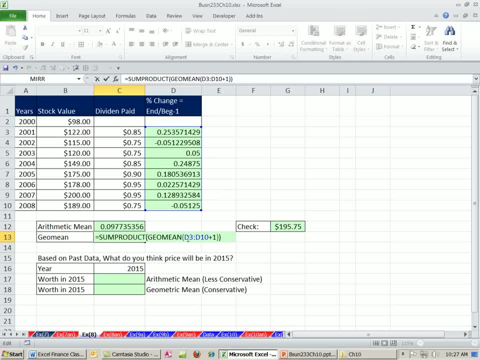 handles arrays. So even though GeoMean, we can see that it calculates to that 109, we have to put it inside of here so that Excel can add it. Now that's going to give us 1.09, and we would need to subtract 1 from that. 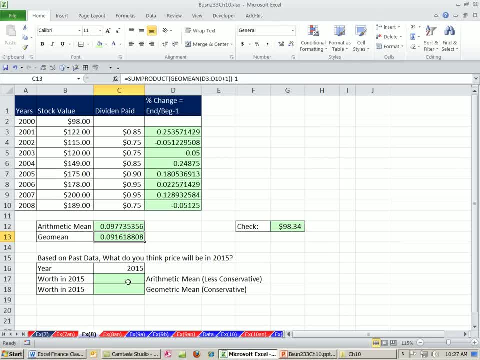 So there's our GeoMean, There's our formula. Now we can estimate Less conservative and more conservative. So we'll start with this one. We'll say, hey, here's the ending value in 2008.. We're going all the way till 2015.. 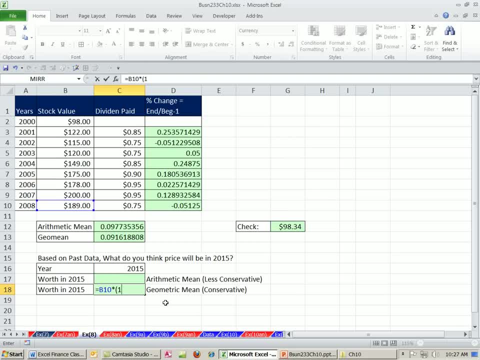 So I'm going to say- hey times in parentheses- 1 plus our geometric mean. This is the true, This is the true average compounding rate that we should use, And we have to raise it to a number of periods. Well, I haven't specifically calculated that. 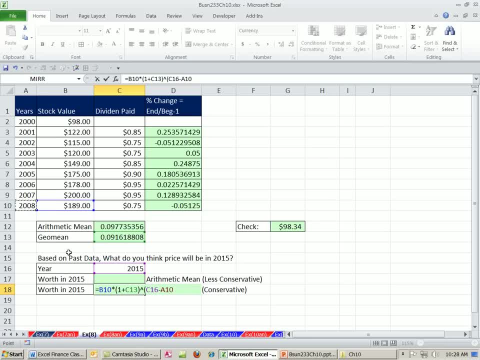 so I'm going to say the year 2015 minus 2008.. That'll calculate to our number of periods, And so there's our expected return based on this past data. So we've estimated, that's the average. Now let's go ahead and do the same calculation. 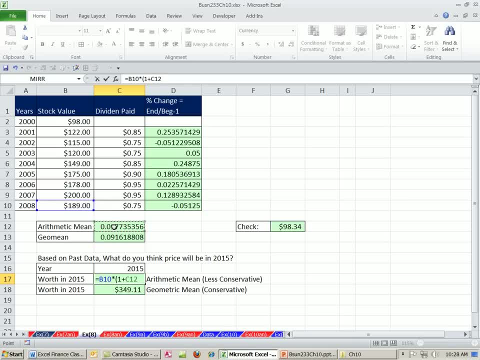 but use the array Arithmetic mean. Notice, the arithmetic mean is always going to be higher, unless they're all the same, And we'll raise it to the same 2015 minus 2008.. So it's going to give us a slightly larger number. 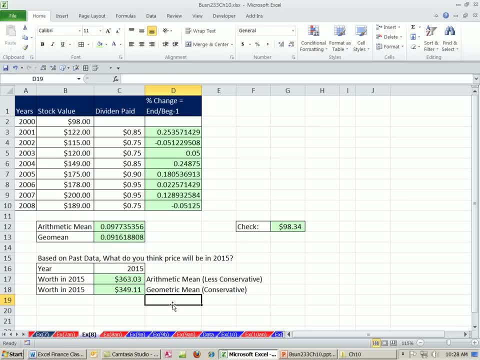 This is going to give us a slightly smaller number. All right, that's GeoMean and Arithmetic Mean. We'll see you next video.